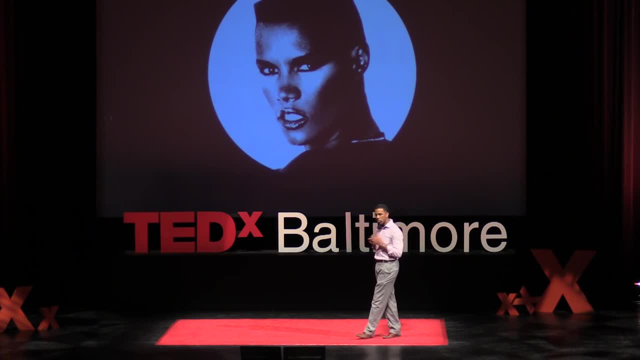 features: the high cheekbones, the square jaw, the pointy chin. These things are dictated by the structure of the underlying facial bone. Our facial bone determines our appearance, It determines our sense of self, And when that bone becomes damaged it damages our. 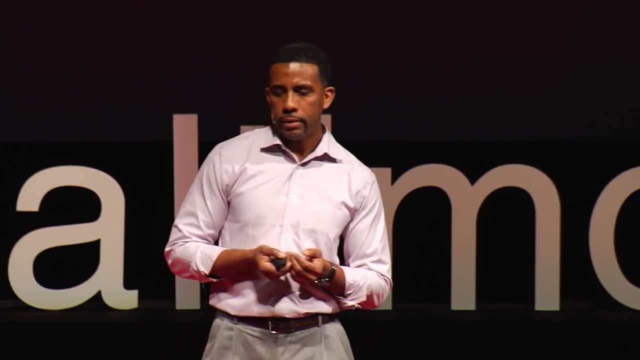 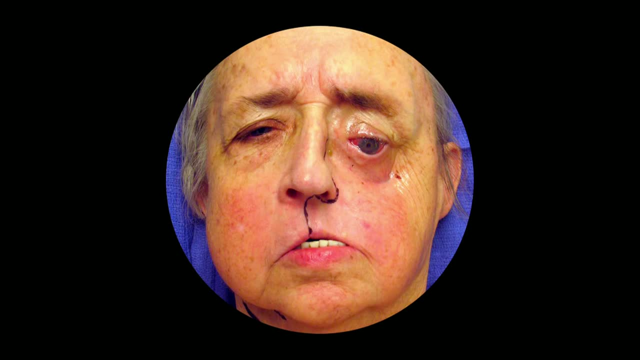 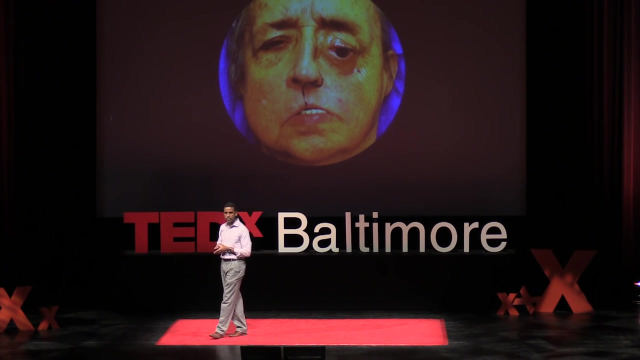 sense of self. Here's a patient. Let's call her Jane. She's an. are you having trouble picturing? today, Jane had a left bone cancer on the left side of her face That had to be surgically removed and it dramatically altered her appearance. 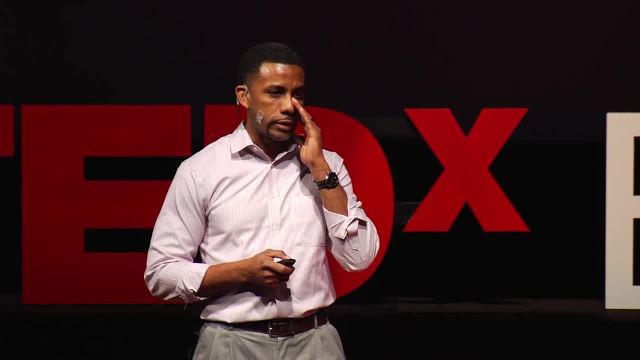 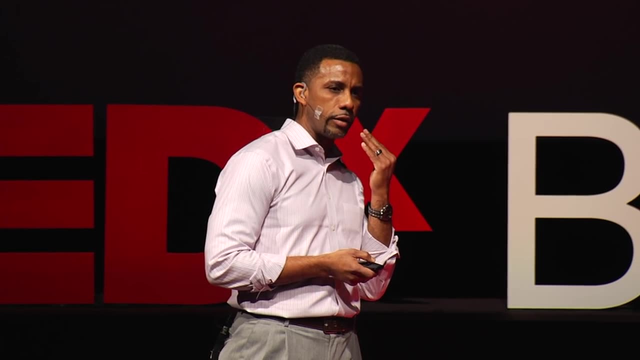 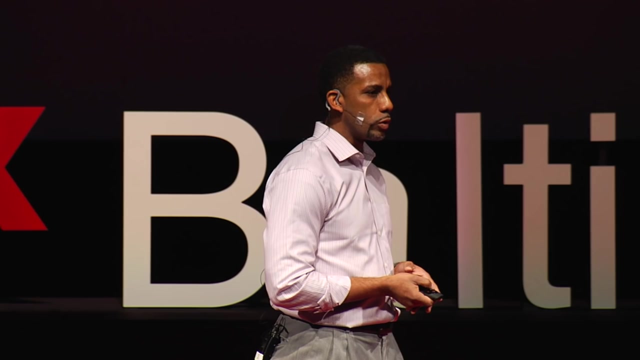 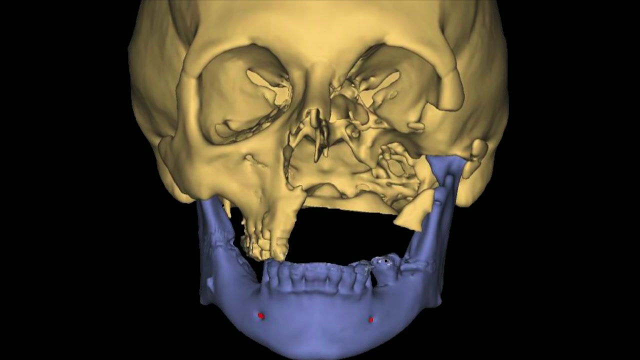 Jane's left eye is drooping, Her nose is indented And that may not be very easy to see right here. her face is also sunken in on the left side. This is what medical imaging shows us about Jane. on the right side, the bone is completely intact. on the left side, that orbital bone that kept her. 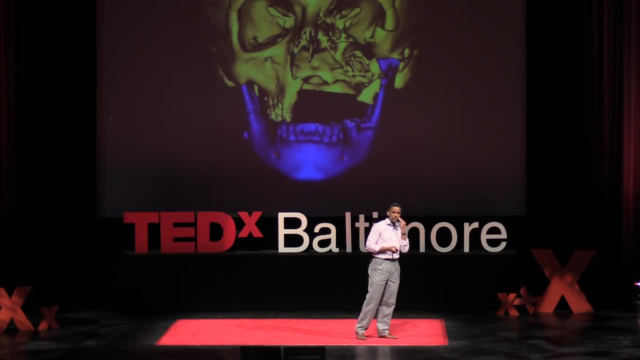 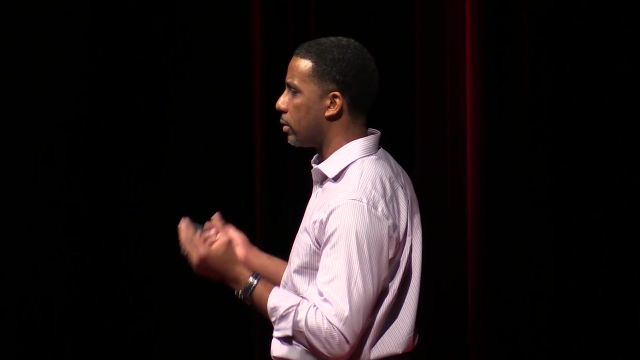 eye in place has been removed and thence her eye is drooping. the entire mid-facial bone had to be removed, hence it changes to her appearance in her nose and her face. a patient like jane is going to require a bone graft to to reconstruct her face, but she's not unique. every year within the united states, there are up to 200 000 people who require bone grafts for skull and facial reconstruction at a health care cost of up to one billion dollars. so let's imagine someone like jane who's living in united states, one of the most technologically advanced countries in the world with access to. 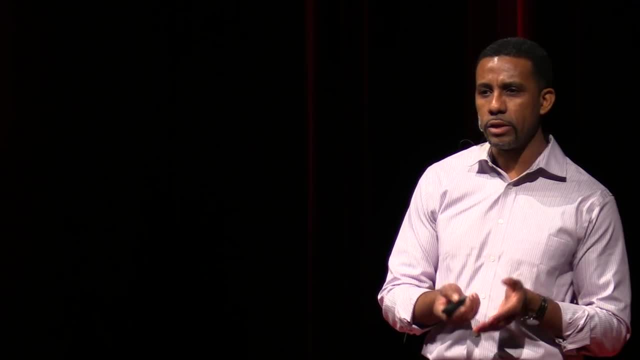 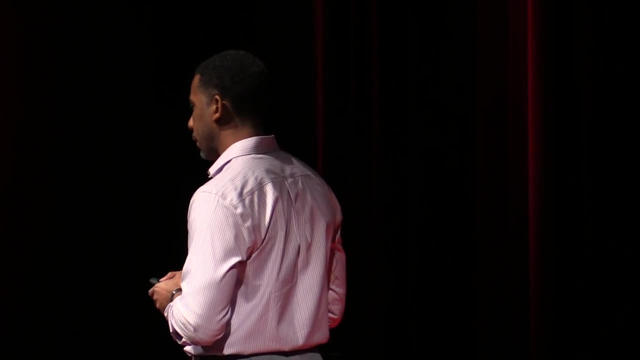 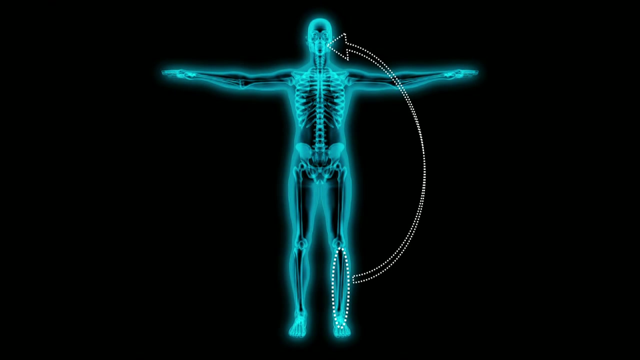 the best healthcare services in the world and she's not unique. she's not unique. she's not unique with access to the most talented surgeons. how would she be treated? this is how they treat them currently. this is a state-of-the-art treatment. it's called autografting, where i'm going to take a bone from another part of your body. often it's a leg bone. 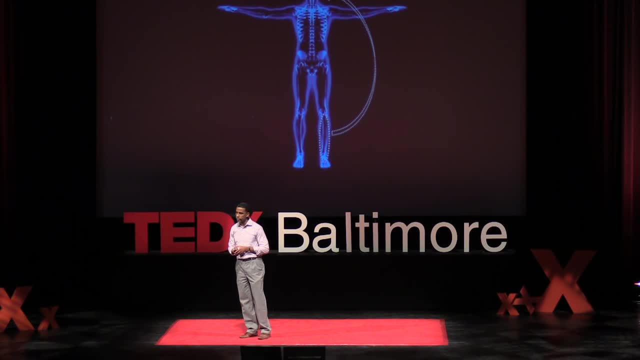 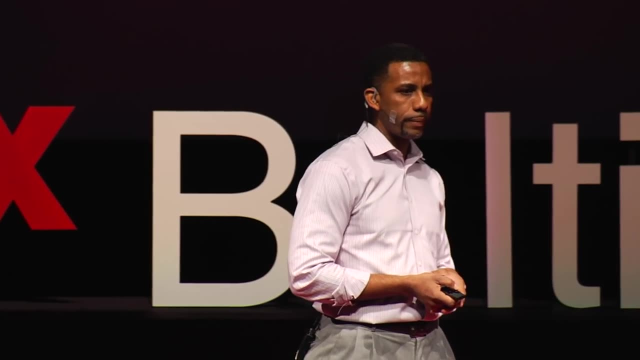 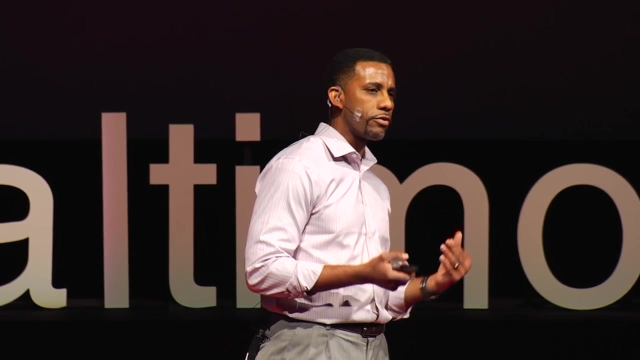 and i'm going to transplant it into the facial region. this is what jane looks like during surgery or surgical planning. that leg bone has been broken up into four different pieces and reconstructed like a puzzle, trying to put it back, to reconstruct that facial appearance. this is going to. this is going to result. 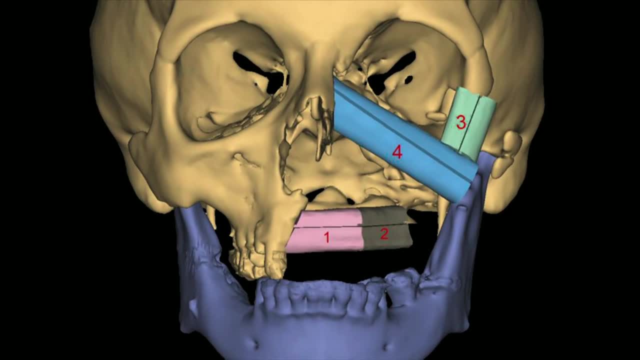 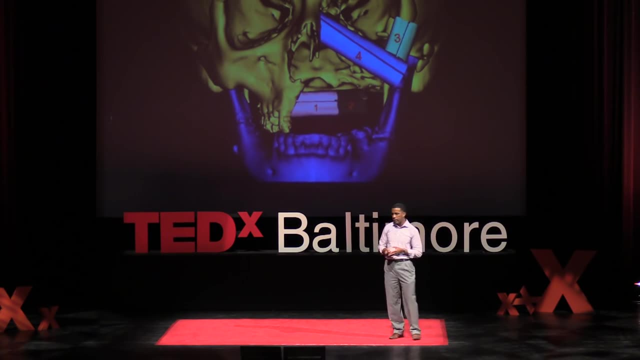 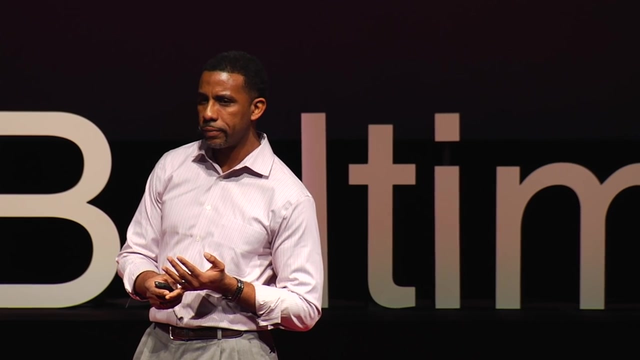 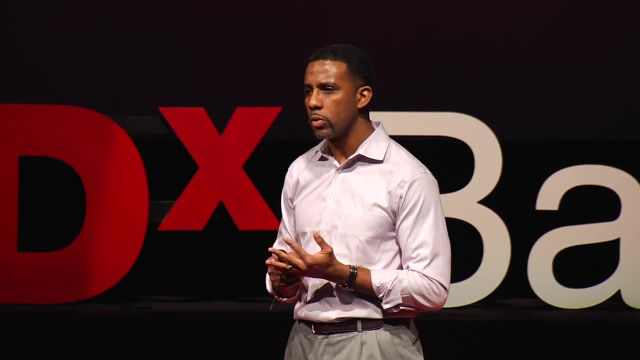 in a marginal improvement in jane's appearance and i've come to believe that this approach is primitive. i, together with my colleagues, are working on an approach to regenerate bone that has the appropriate anatomical structure, that is, a living tissue, so that the patient grows and changes. that bone grow and change along with the patient. 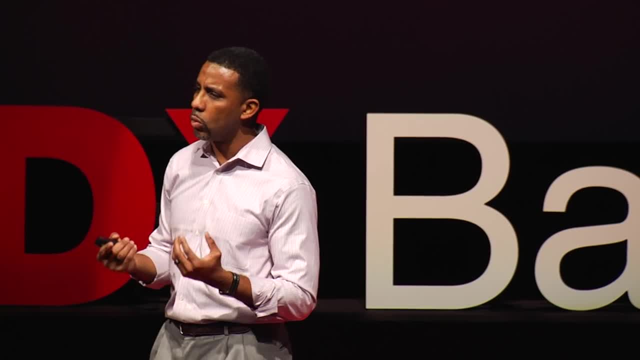 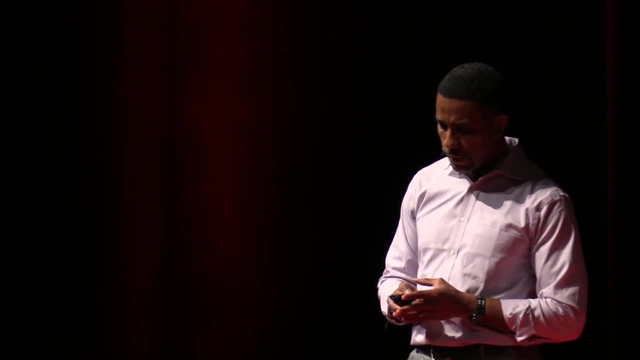 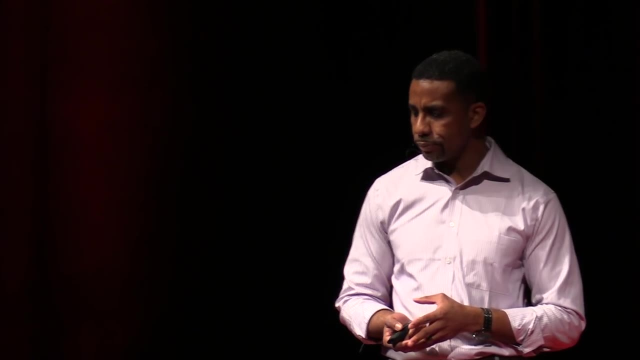 but also that bone should be comprised of the patient's own genetic material so that it doesn't have any rejection, doesn't suffer from any rejection. we call this approach tissue engineering. tissue engineering: we start with a scaffold and that scaffold is very important, so its scaffold is going to determine the exact shape of tissue. 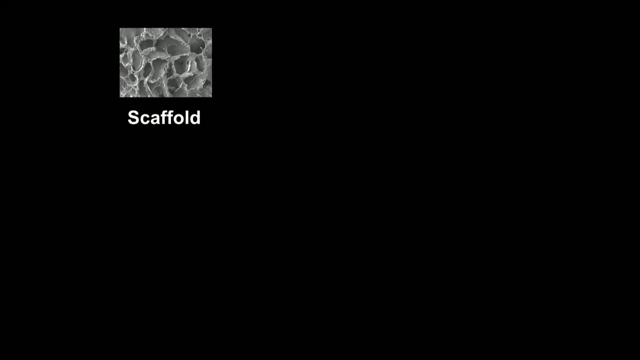 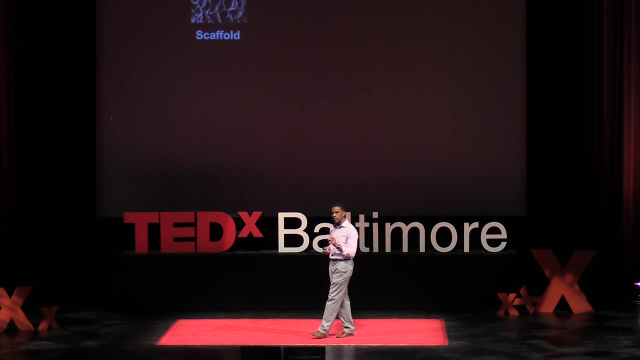 that is going to regenerate, And so we make that scaffold in the exact shape of the bone that we would like to regenerate in this patient. The scaffold is also porous, And what that does is allow cells and blood vessels to grow inside of it. 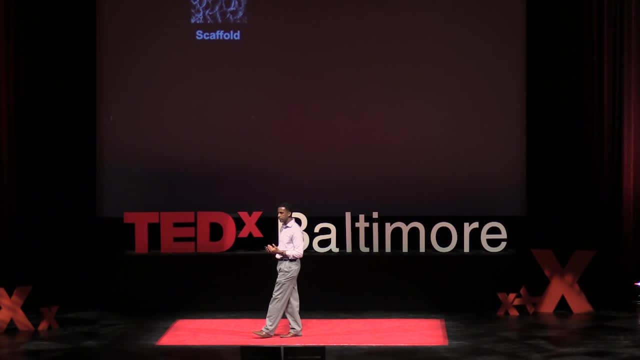 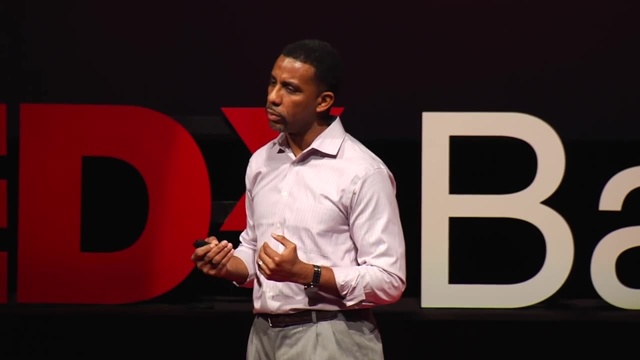 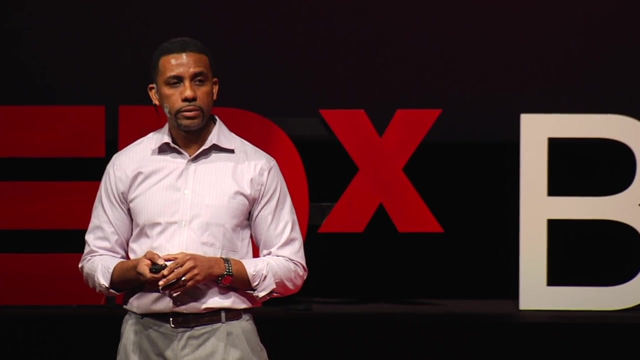 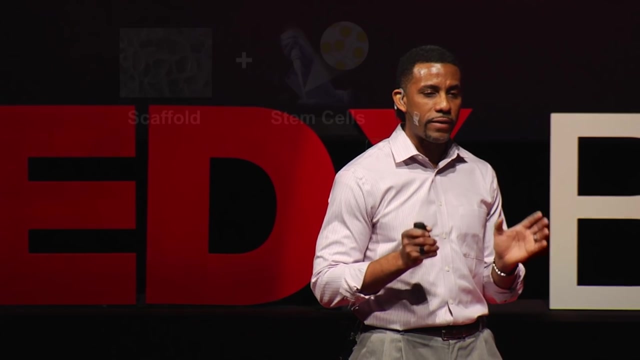 So it can form living tissue, healthy tissue. But the scaffold has another really critical feature. Once that new bone forms, that scaffold should degrade away, Leaving only biological tissue. To that scaffold we are going to add stem cells, The stem cells we get from the patient's own fat tissue. 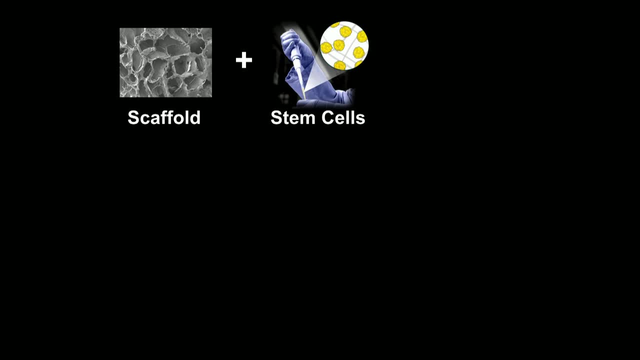 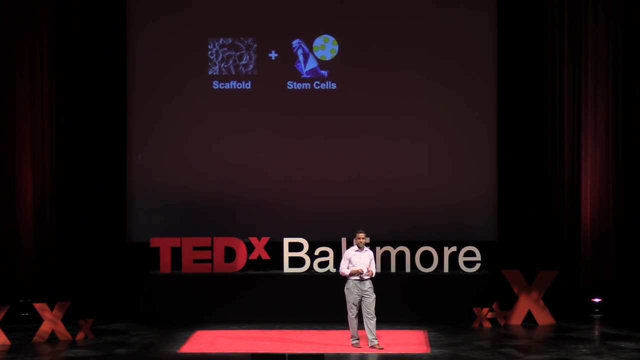 Fat tissue. So for those of us with bare guts love handles, this is our evolutionary advantage: We can take those stem cells and isolate them in the bone. And we can take those stem cells and isolate them in the bone And we can isolate them from that fat tissue. And we keep it in a solution. And that solution we're just going to take and drip onto that scaffold So that it spreads uniformly throughout, So that when the cells go they can form bone throughout that entire scaffold tissue. But the cells have an important characteristic: 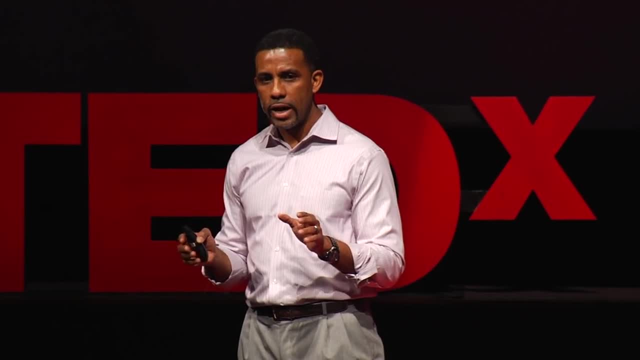 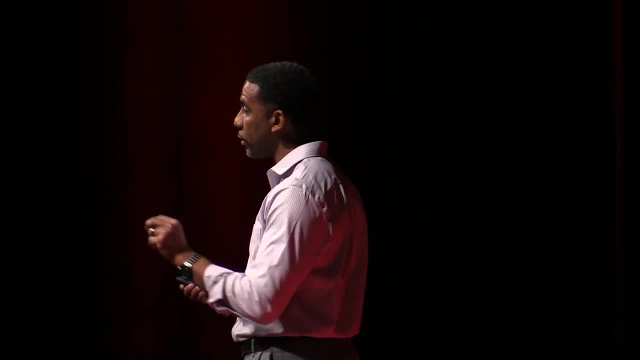 Stem cells can form different types of cells within the body, And so it's important that when you put those cells inside of that scaffold, we give them the appropriate signals so that they know they should be able to do it, And so they can form bone and nothing else inside of it. 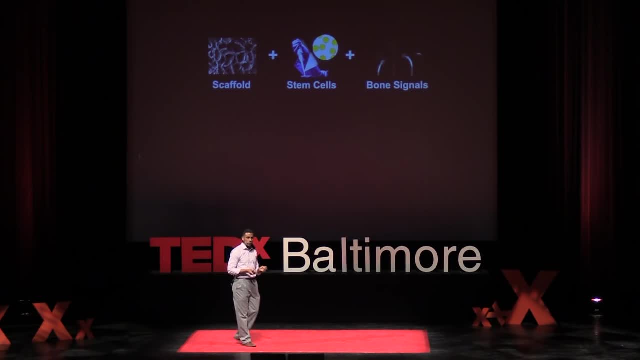 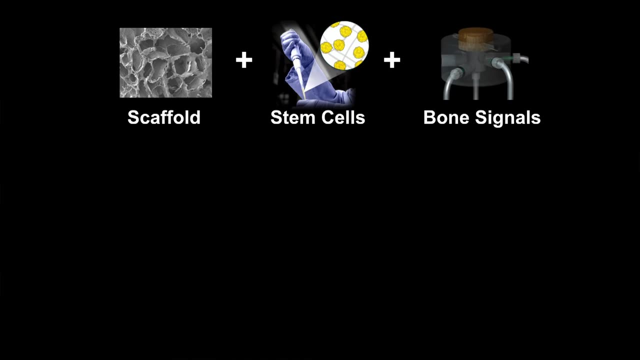 And so we add to those stem cells and scaffold, we add bone signals. We had done this in the lab several years ago. We tried to combine all three of these features: the stems, the stem cells, the scaffolds and the bone signals. 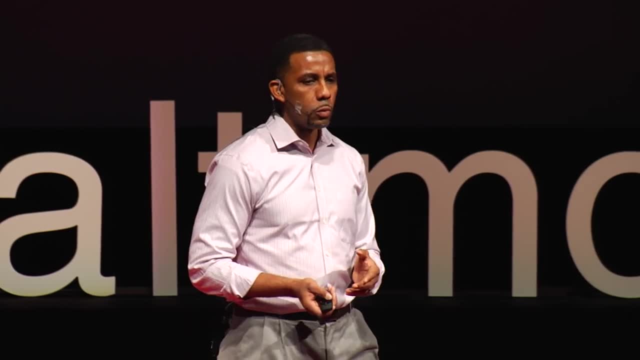 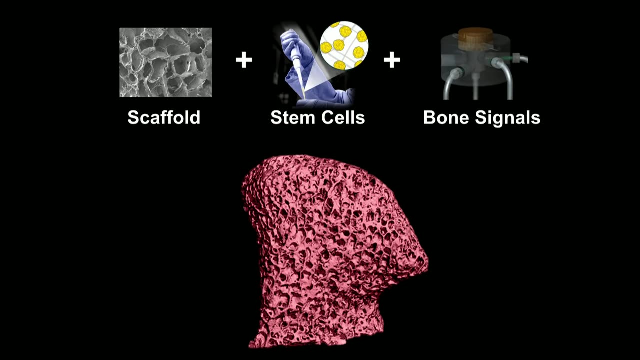 And what we showed was that after a period of five weeks, we were able to grow piece of jawbone. This is the piece that is right at the top of the jaw. This part is in front of the ear. It's what allows us to open up the jaw. 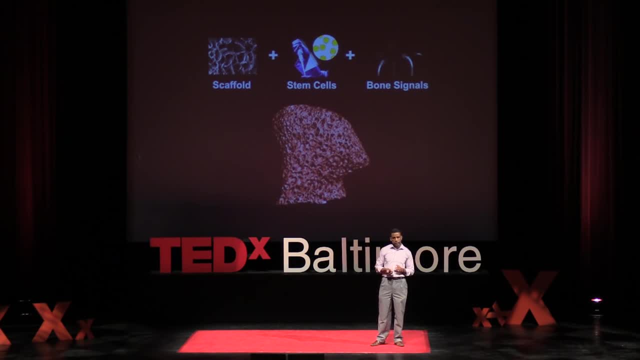 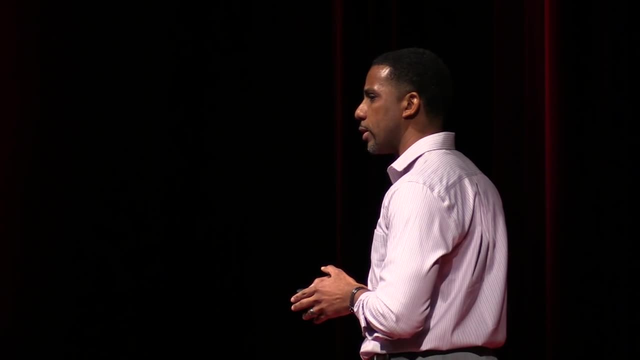 This is the piece that's right at the top of the jaw. open and close our mouths for speaking and for chewing, And so we thought if we could regenerate a piece of jawbone in the lab outside of the body, the next logical step is to see what we can do inside the body. To do this. we work with mice Now. mice are interesting in that they regenerate really well, And so for us to test this within mice. what we did was to create two holes in the skull of the mice, taking very good care not to damage the underlying bone, the brain tissue. 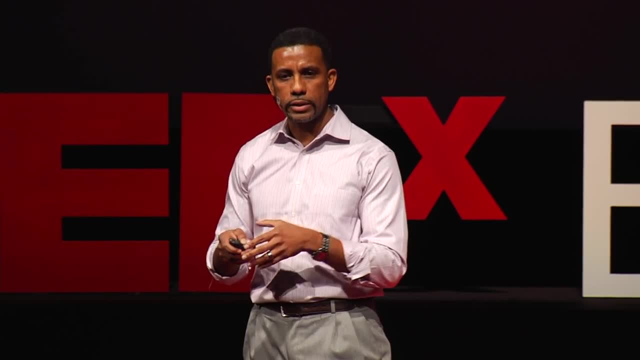 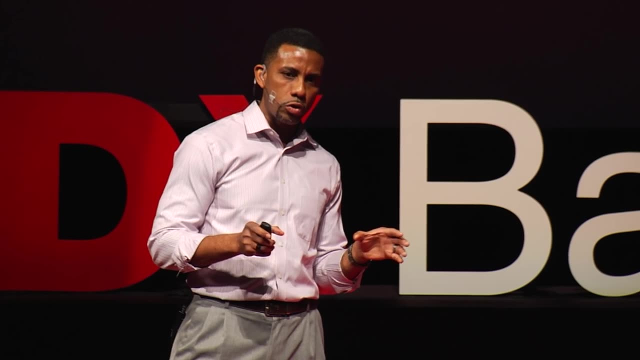 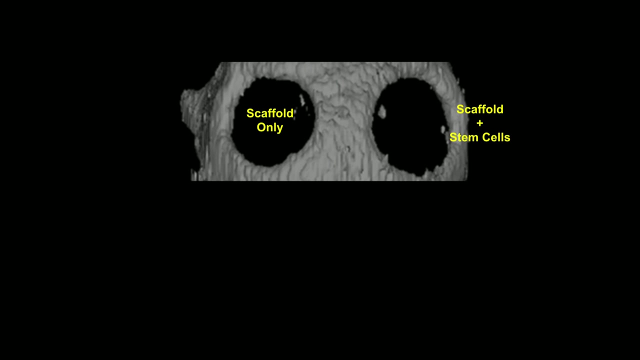 Within those holes. what we did was to put scaffolds and stem cells and bone signals. This is a CT image of the mouse that shows only the bone right, so it's like a CAT scan for mice. On the left side you can see the hole that we created, one of the circular defects that 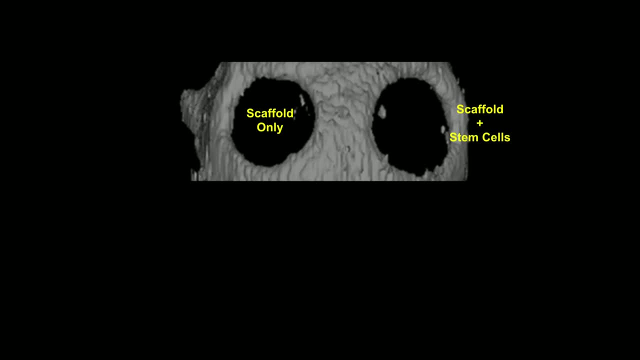 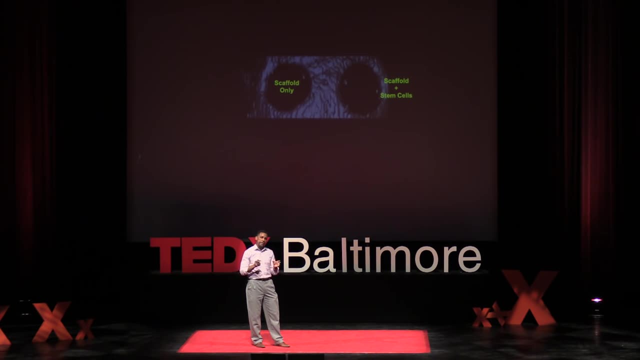 we created that has the scaffold only inside of it. On the right side we've put the skull, We've put the scaffold and we've populated that scaffold with stem cells And you can start to see the beginnings of some bone forming inside of there, shown by: 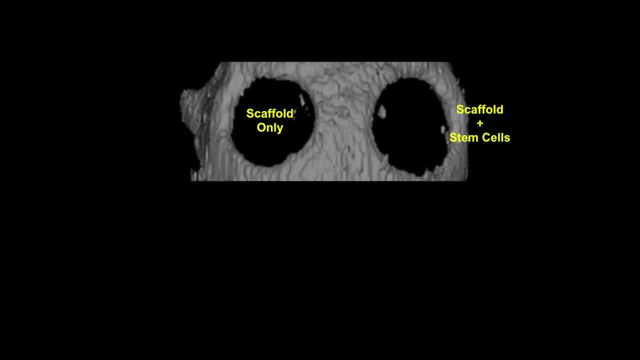 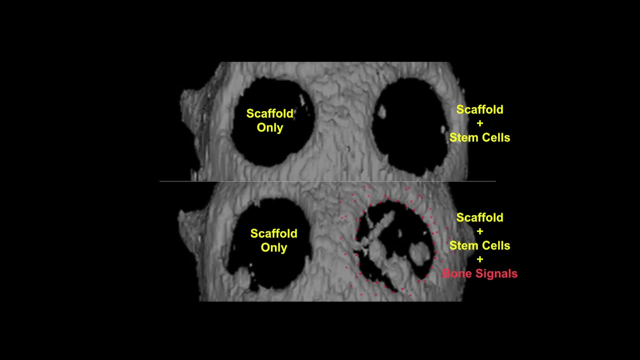 the little nodules that you see on the inside of the circle. However, once we add those bone signals to that defect, we see a dramatic difference. We can regenerate large quantities of bone within that defect after a period of six weeks. That new bone that's forming is taking the shape of that scaffold that we've implanted. 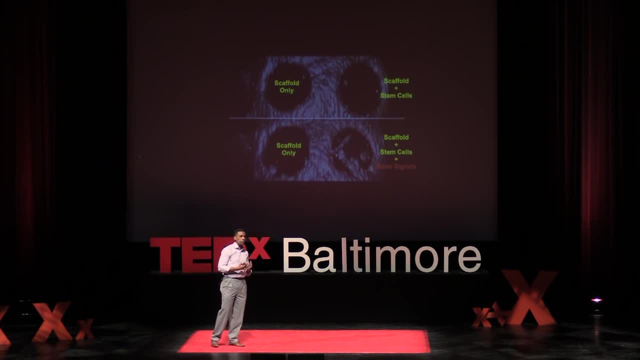 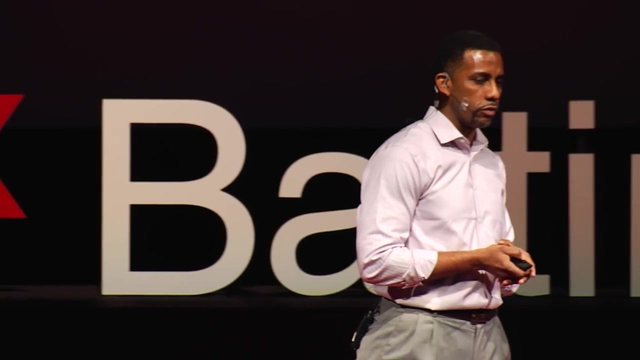 inside of that defect, And so forth. So for us, what we feel is that we have the fundamentals of a way to revolutionize the way that patients like Jane would be treated when she comes to the clinic. So how would that change the way that Jane is treated currently? 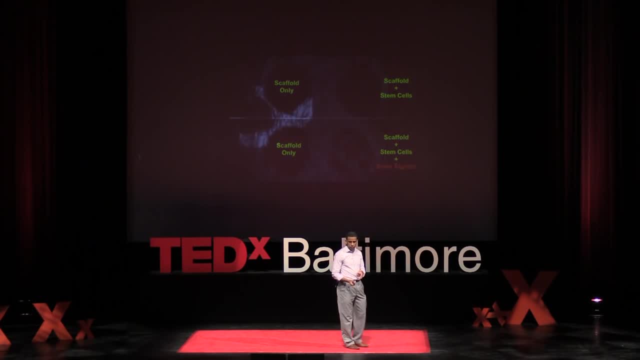 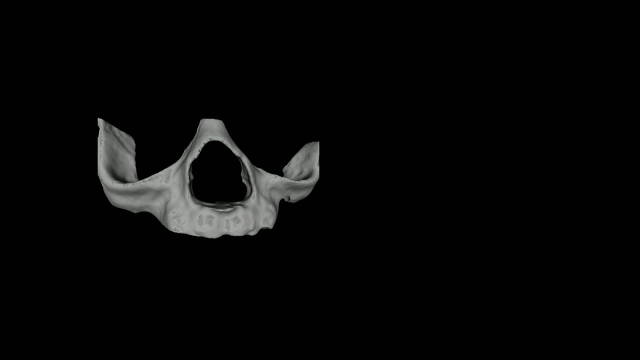 Currently, we would take a CT image, as we've done before, of this patient. So the surgeon would take a CT image when the patient comes in. What if the patient is missing bone? Well, we can digitally include that, And so, at the end of this, whether it's a cancer patient or someone with a congenital 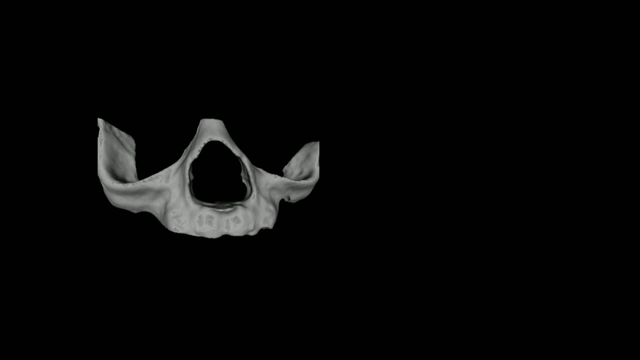 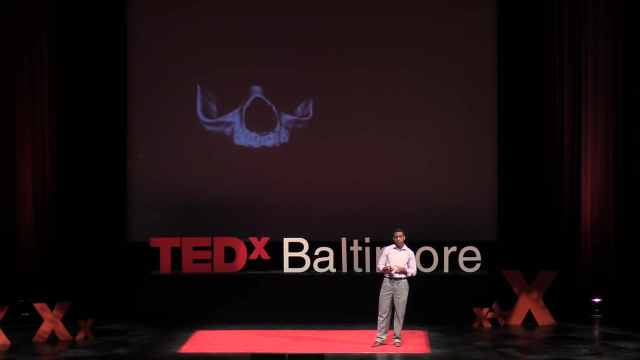 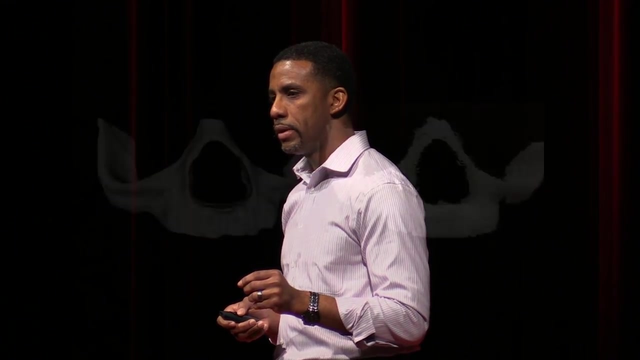 defect, who never had bone in that place. we can still render what that three-dimensional bone volume would look like. With that three-dimensional bone volume, we can take it and we can 3D print scaffolds in the exact shape of the bone that we're trying to regenerate.